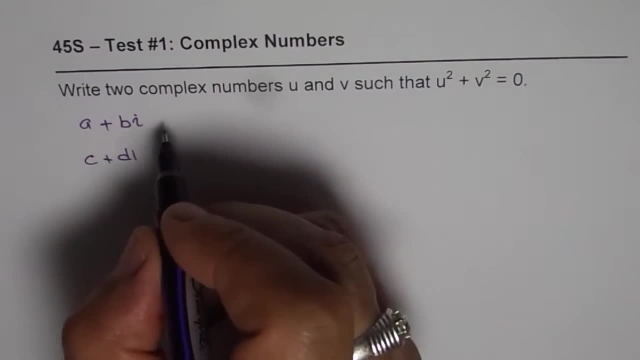 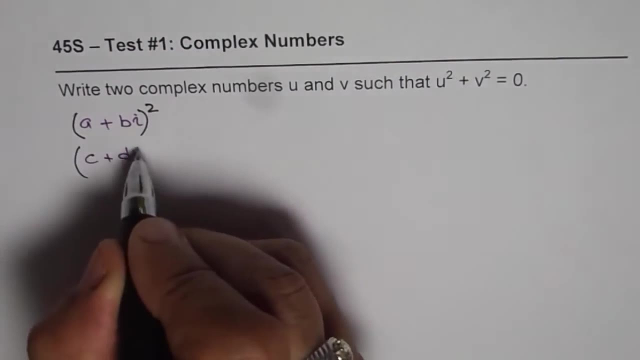 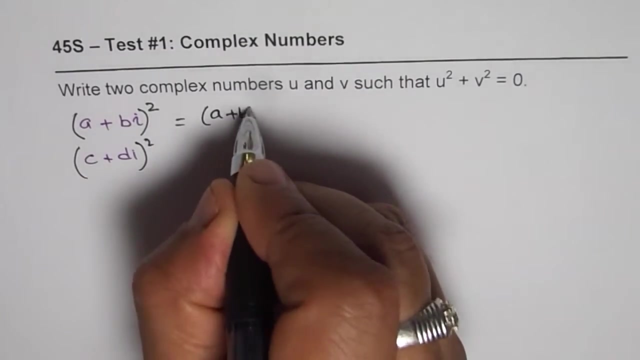 Then what will be the square of these? Then the squares will be: let us figure out squares of these numbers will be like this: correct? That means you are going to multiply the number by itself. So we get a plus bi times a plus bi, correct? 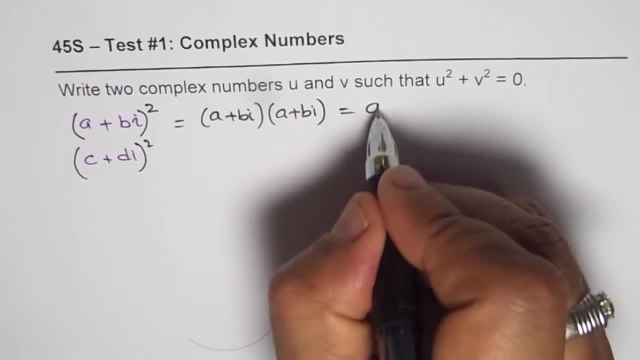 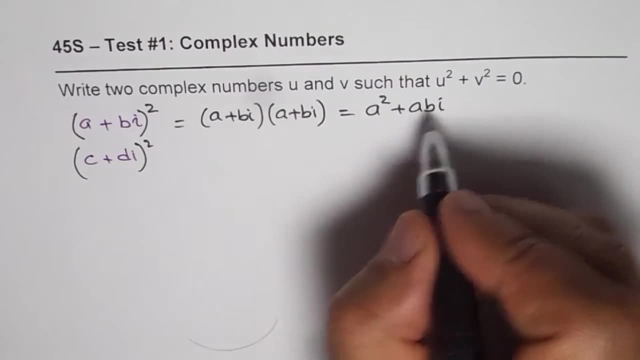 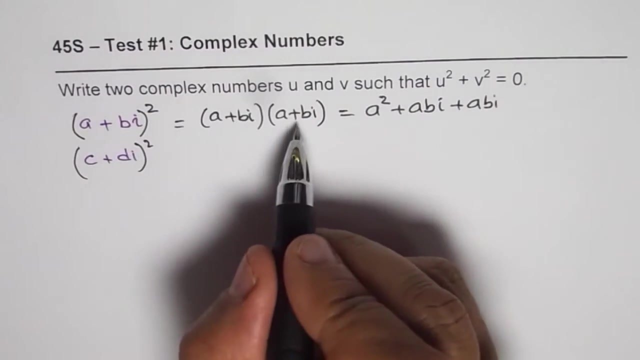 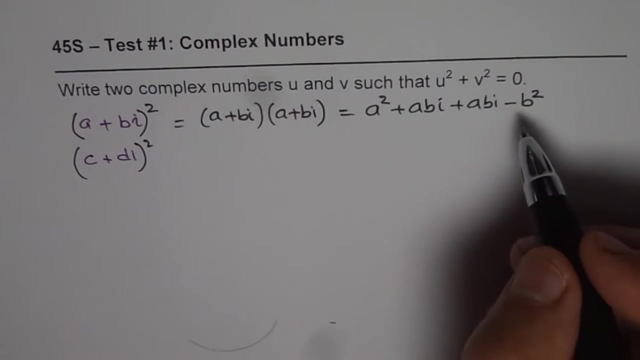 So when I multiply, I get a square, a bi, plus a bi again. And when I multiply I get plus b square and i square, which is minus b square. right, So I am just cutting short by one step. It should be b square, i square. you know, i square is minus 1.. So I wrote this negative, correct. 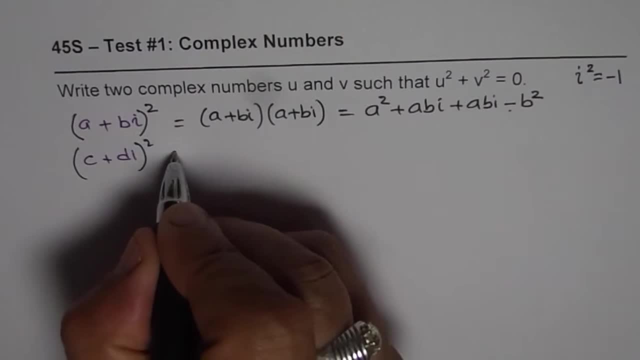 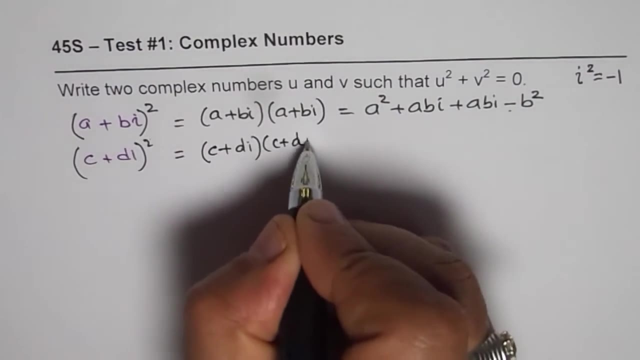 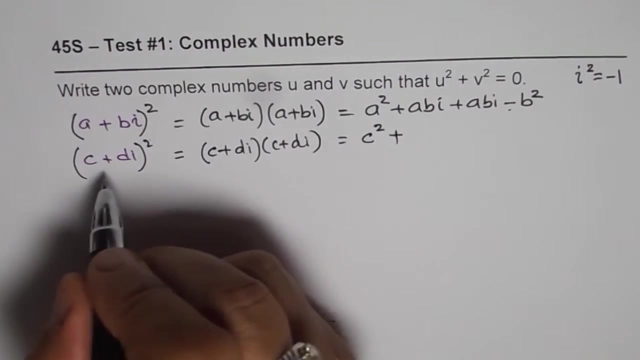 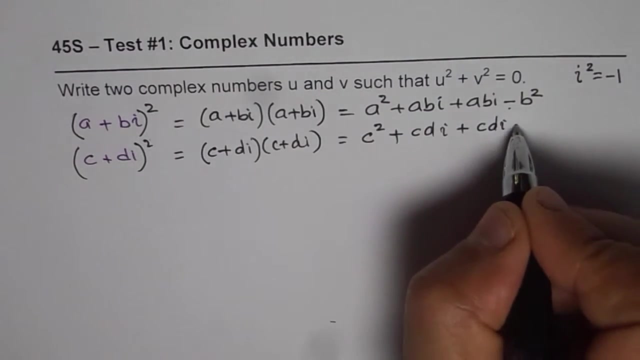 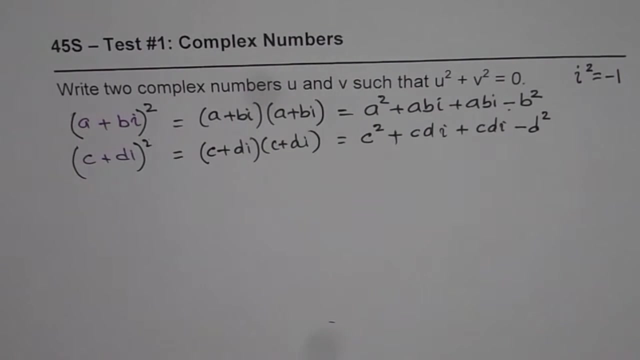 So at this stage I think we can do that right. The second one is c plus di whole square. So the same thing, c plus di times, c plus di, and when you square it you get the same thing, which is c square plus cd. i plus again cdi minus di whole square, which becomes minus d square. So you get the same thing. 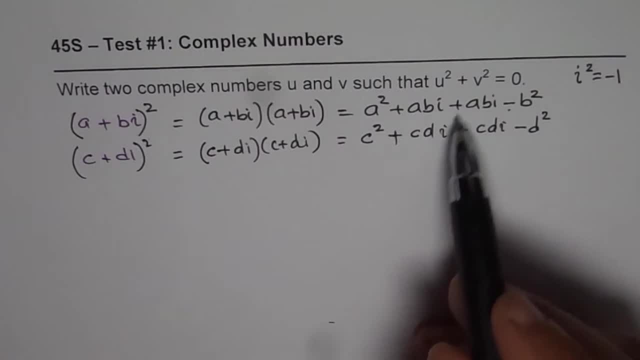 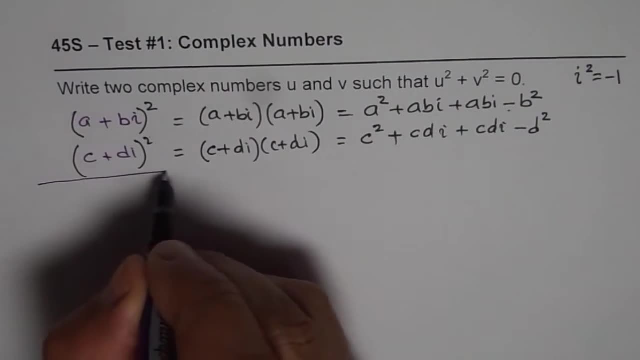 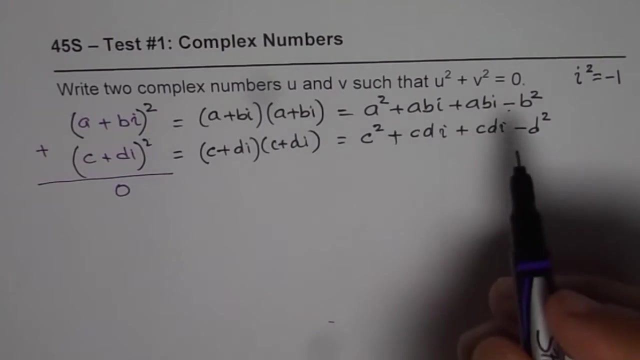 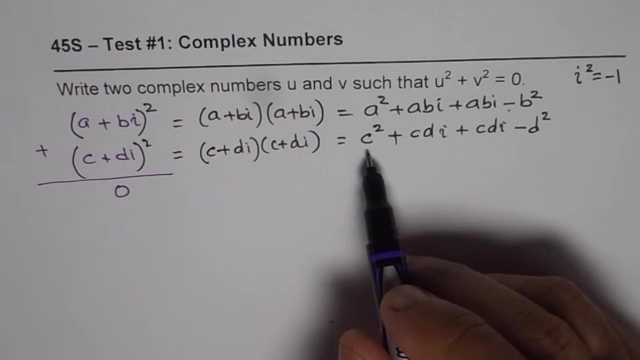 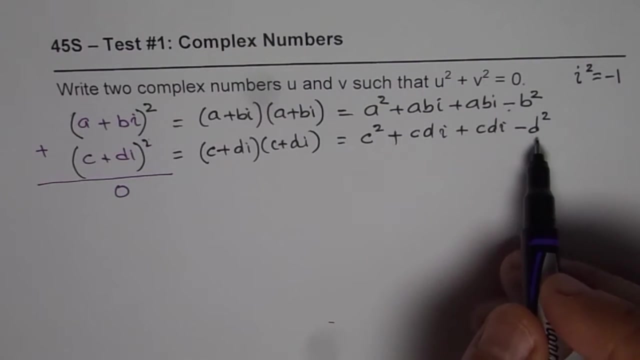 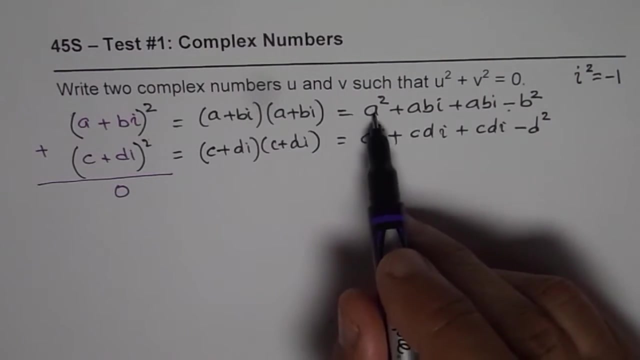 Now the question is: when you add these two, when you add these two, you should get 0. That is the question. The question is: if I add these two, I should get 0. That is the question: How to find these two. Now, if you compare these values to make it 0,, what should we do? We should make: if I make d as negative of b, then can it work? No, But if I make d as a, I hope it will work. 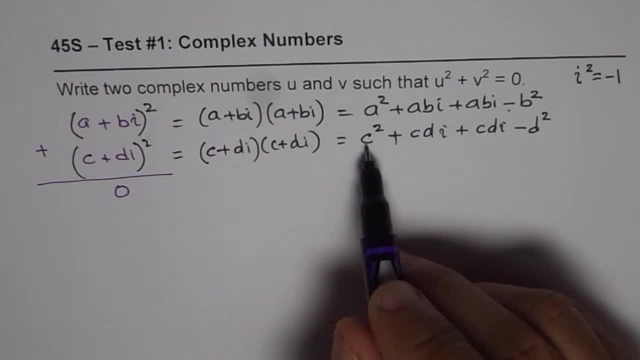 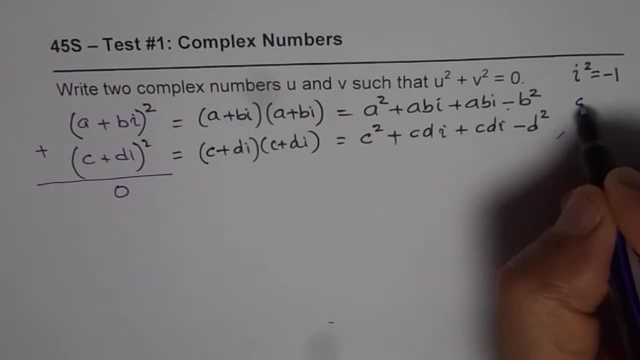 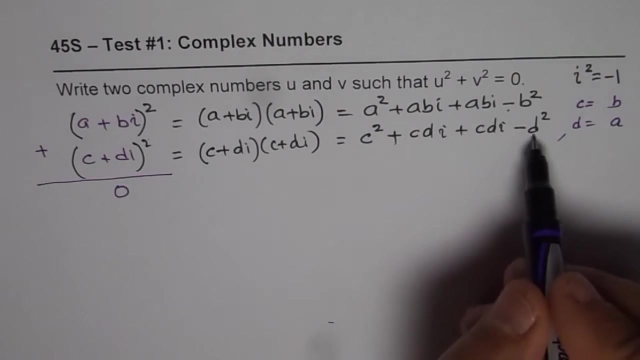 There is minus Right And c as b, then we get minus here, right, c as b. So think about it. So if I make c equals to b and d equals to a right, In that case I'm able to actually cancel out these two. But then how will I cancel out these ones? That is kind of tricky. So what I can do is one of them I can make negative, That is. 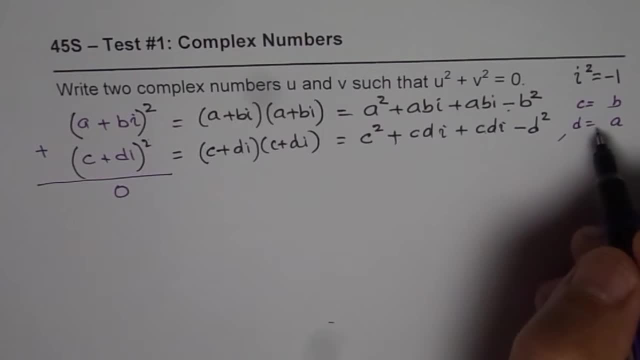 I could have one of them as negative. In that case I'll get negative numbers here and then they will cancel out Right c times d, c times d will be ab. So they will add up To get them cancelled off. one of them should be negative. So let me make any one of them negative. So I'll make d negative, okay, d negative of a. So that is kind of learning from our equation. And then 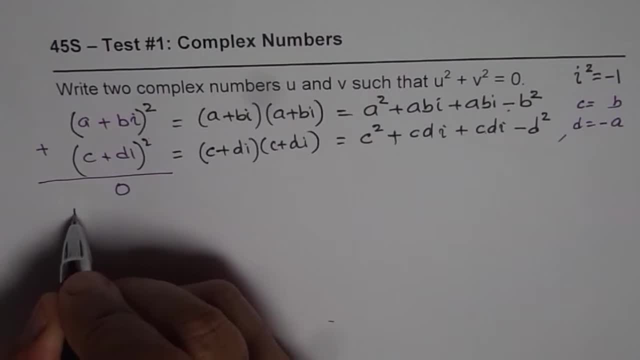 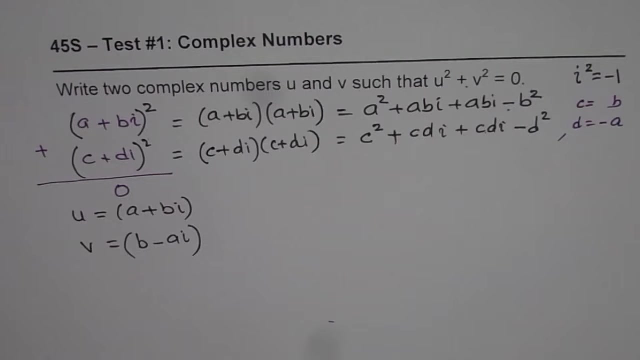 we'll try it out. So we say, let u be equals to a plus bi and v be equals to, instead of c plus di. I'm changing c as b, So I'm writing this as b, And d is minus a minus ai. Then I think some of the squares will be zero. So these are my values for u and b, Correct? So that's my answer. 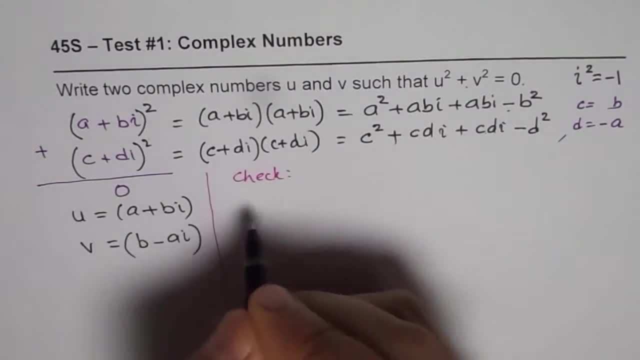 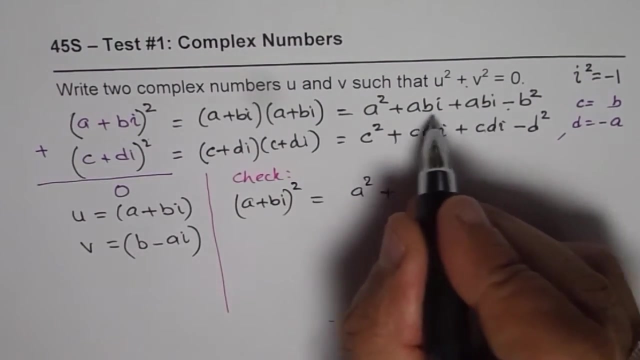 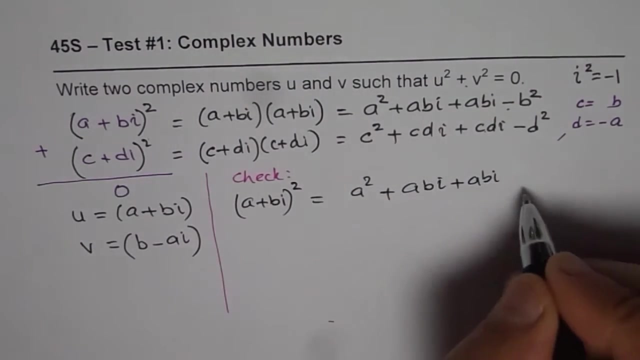 Now what we will do is: we'll just check whether it works or not, Correct, So let us do a plus bi. whole square is already known to us, which is a square plus ab. We'll write a square plus. I'm not combining them on purpose. right, I could write two times abi, but let it be like this: Plus abi minus b square. Now what is b minus b? 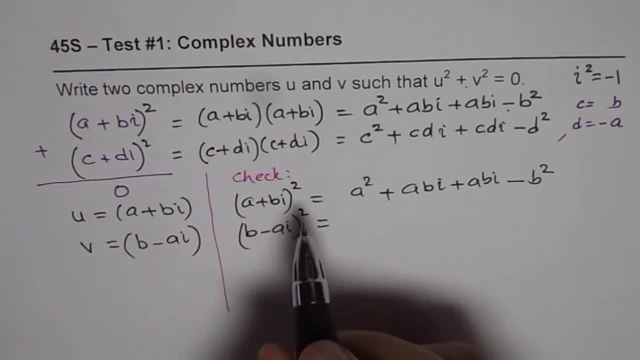 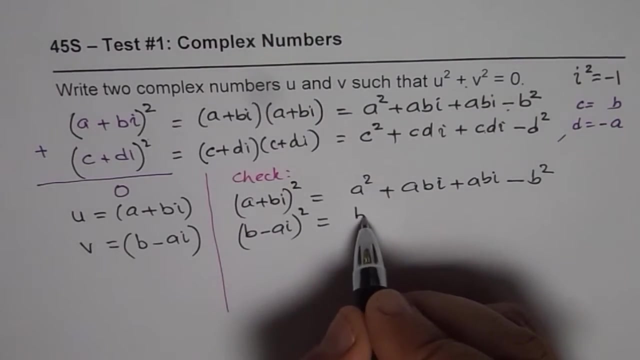 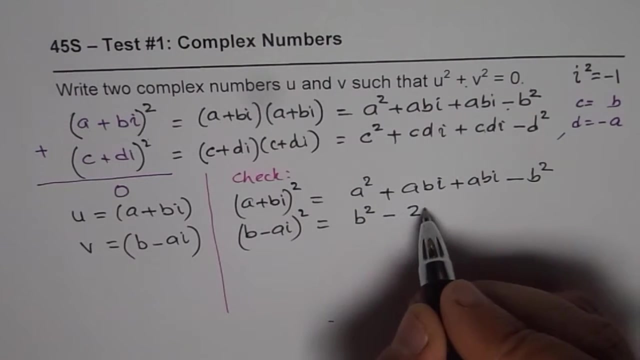 b times ai, So that'll be b times ai, right? So we'll have to multiply this two times, So that'll be. you can use the quadratic formula also, Correct. So b square, which is the first term, minus two times both, which is minus two times ab or bi i plus this one is: 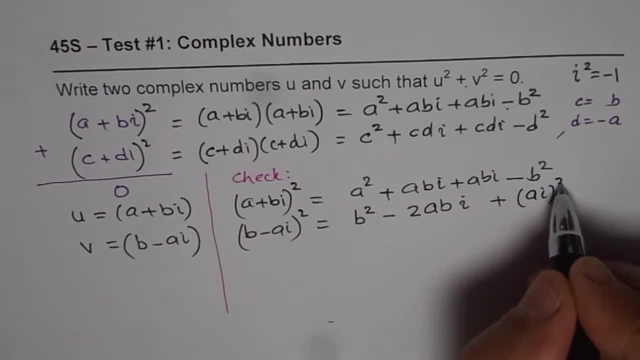 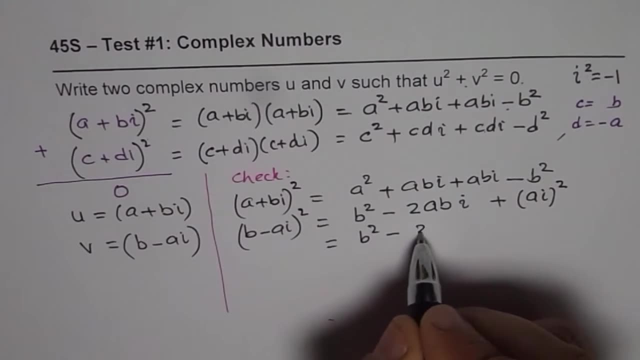 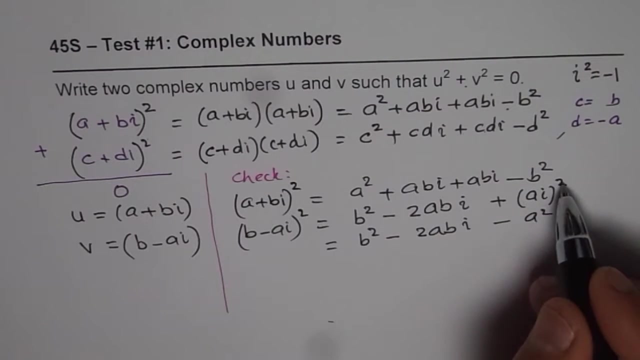 square of ai. So ai whole square. That is what you get. Now let me expand this one. So b square minus two abi a square is written a square, but i square is negative, So we get negative a square, Correct? Now if you look into these two equations and add them, then b square minus b square do you see that They cancel out? 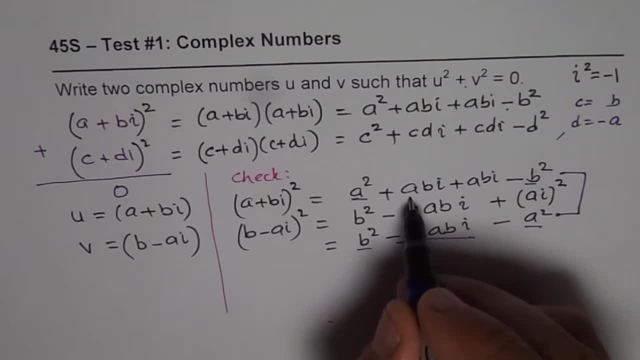 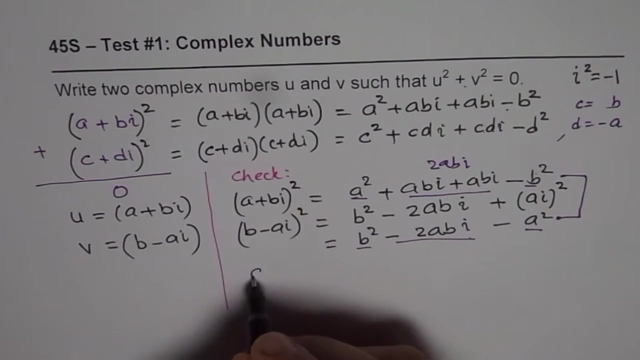 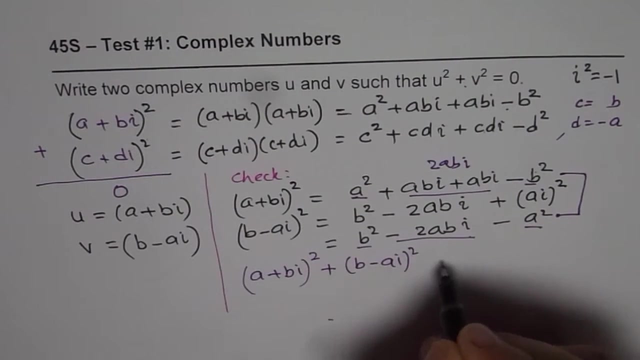 Minus a square, cancel out. Minus two ab. So plus two ab, This is plus two ab, Right With i. So they also imaginary parts, also cancel out, Do you see that part? So it becomes zero. So what we verified here is that indeed, a plus bi whole square, plus b minus ai whole square is equal to zero, Right? So these are general. 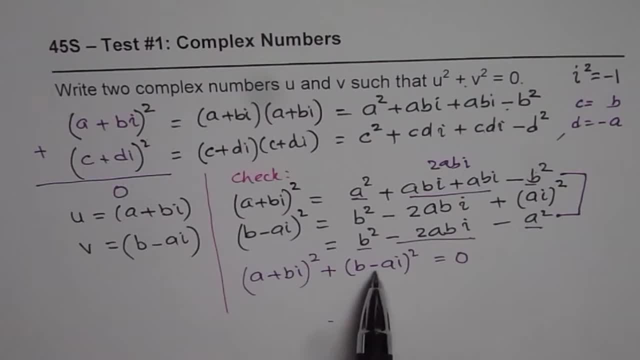 complex numbers, And that is how you can get two complex numbers whose sum of squares is zero, Right? So the answer I could write- let's be specific. We say two plus i whole square. sorry, is the first number, And let this be. u equals to u And v for us will be now one, right? This value is one, So we'll write one minus two i, Is it okay? 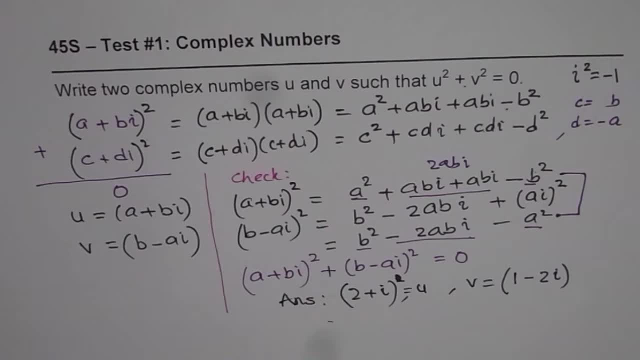 So that becomes the other variable. So in the simplest form, this is a good example to give. So general value is any variable. So what we do is we swap the real and the imaginary term and change the sign. You could make either b minus or a minus One of them, since we need negative here. I hope that works. So what I'm trying to say here is we could also be. we have to swap minus, b minus a minus. 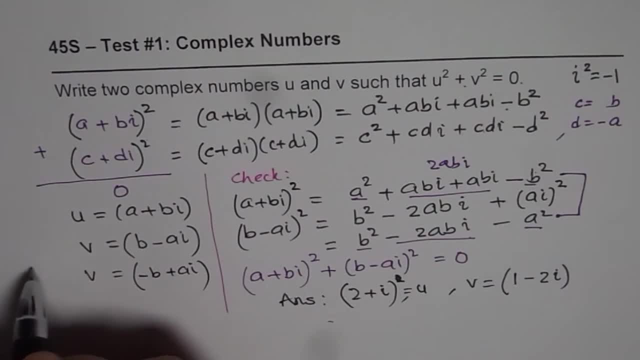 b plus ai will also work Right. So any. So or we can say: or these, So for u. these are my general answers, Right? I hope this general formula helps you to understand how to answer this question. Thank you and all the best. 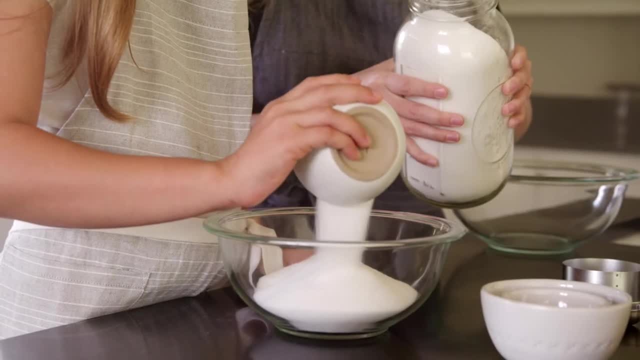 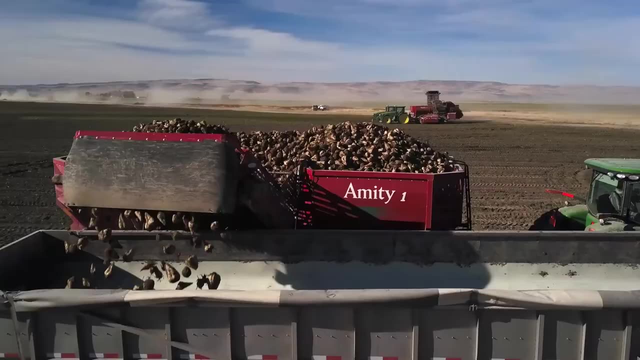 Are simple ingredients important to you. Do you know that the sugar in your pantry and in some of your kids' favorite foods comes from sugar beets and sugar cane grown on farms? Yep, real sugar comes from nature, not a lab. Sugar is about as real as it gets from family.